In 1694, the Bank of England became the first public bank to regularly issue banknotes as an alternative to coins as a means of payment. Three centuries later, it's primarily tasked with maintaining price stability, much like any other central bank across the world. 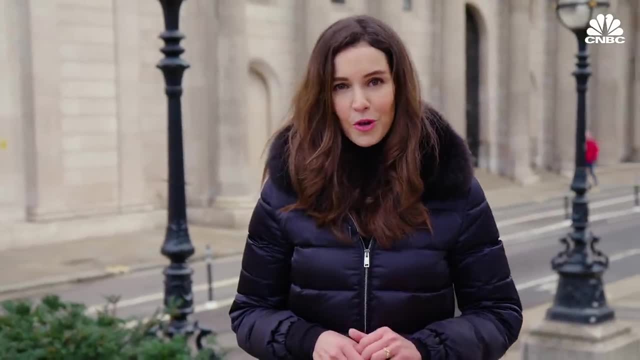 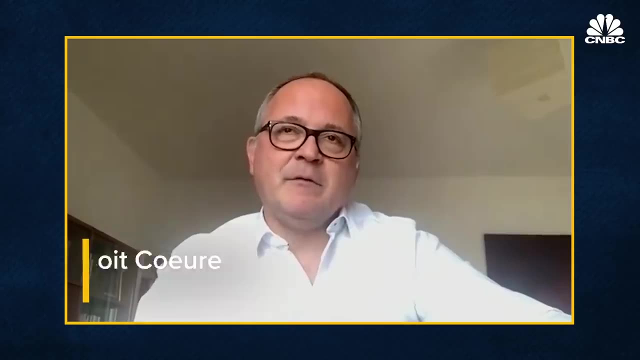 But these cautious institutions are now buzzing with talk of a revolutionary concept, a form of money you cannot see central bank: digital currencies. When you ask central banks around the world whether they are exploring CBDC, one year ago the answer was 80% of them were exploring and now it's nearly 90%. 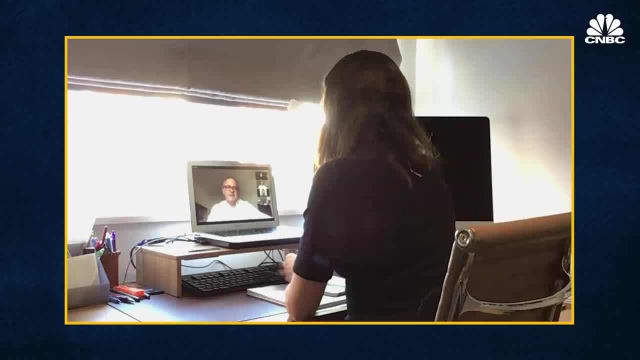 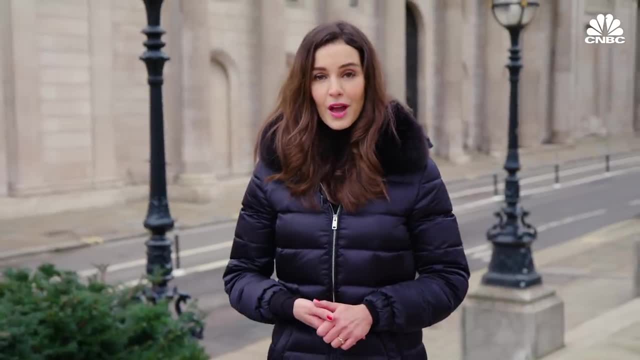 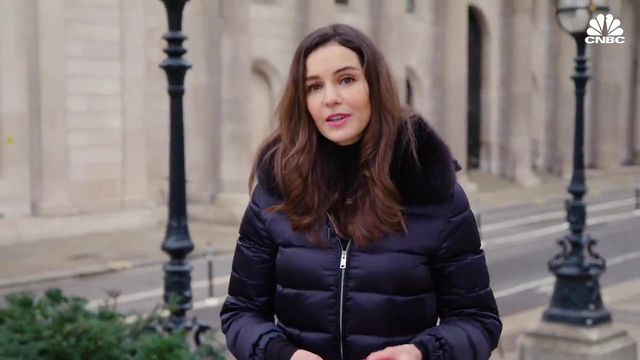 Last year, 40% were experimenting and now it's 60%. The vast majority of central banks are exploring CBDC. The idea of digital money is not new. Many of us use debit and credit cards or payment apps for transactions. But what would make a central bank digital currency different? 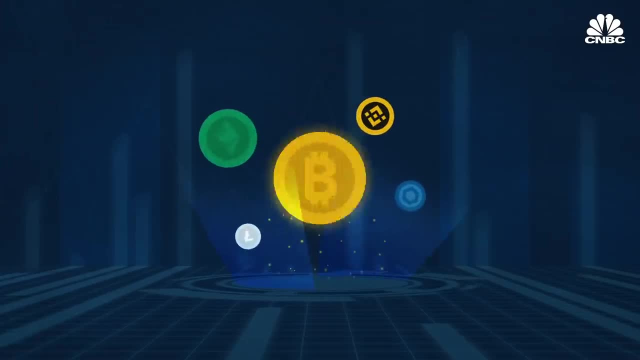 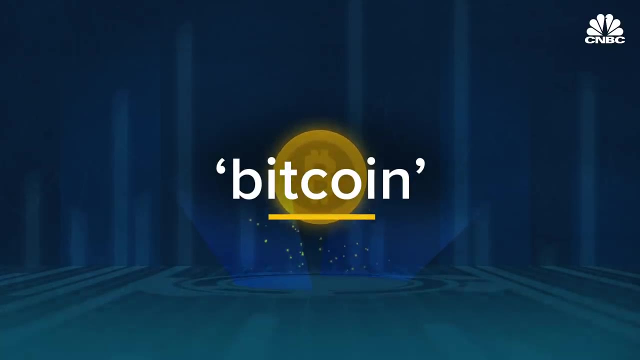 One of the big financial developments over the last few years has been the rise in popularity of cryptocurrencies, with one in particular, Bitcoin, standing out. Following Tesla's announcement that it bought $1.5 billion worth of Bitcoin in February 2021, the volatile 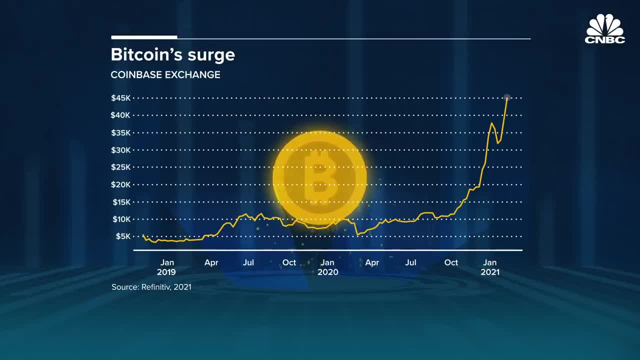 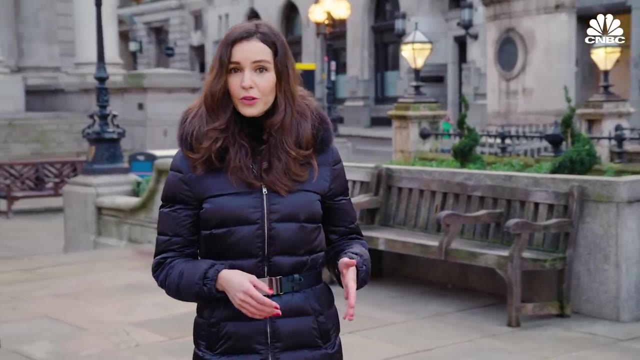 cryptocurrency's price surged to new highs, giving it a theoretical market capitalization that is even larger than the world's two largest payments processing companies, Visa and Mastercard. Unlike traditional money, cryptocurrencies are not issued by a central bank, but rather via a decentralized network of computers. 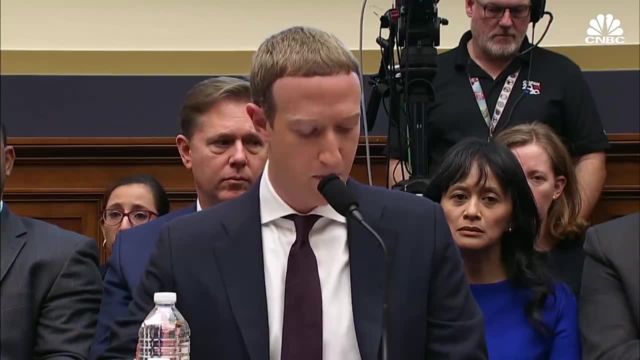 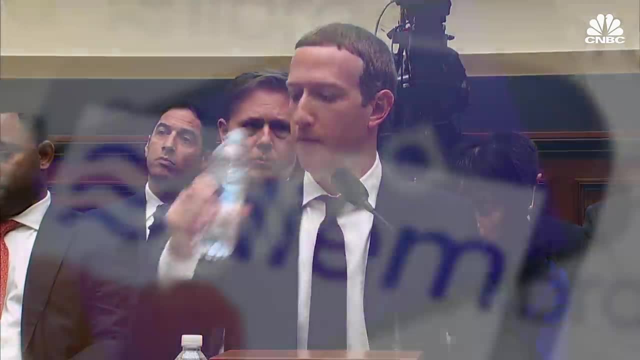 typically using blockchain technology. Even Facebook is trying to get in on the act with the 2019 announcement that it would develop its own digital currency, known at the time as Libra and now rebadged as Diem, And so at that point, central bankers started to realize that they were really. 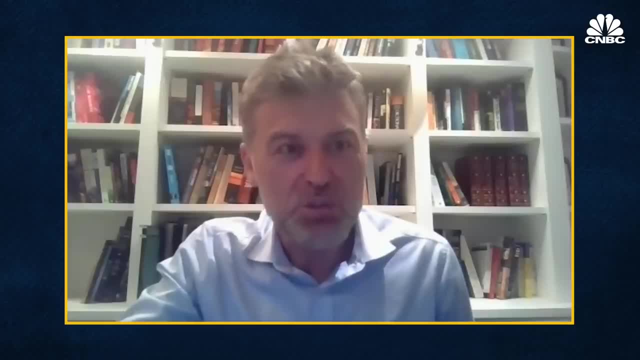 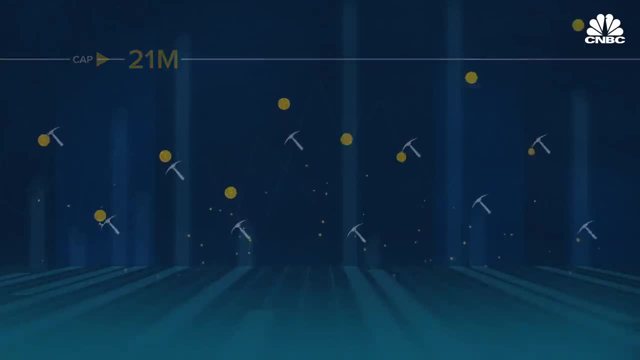 under some threat And the question became: if we can't beat them, do we join them? Investors in Bitcoin believe that, because there is a theoretical cap on the number of Bitcoins that can ever be mined, the cryptocurrency will become increasingly valuable at a time when. 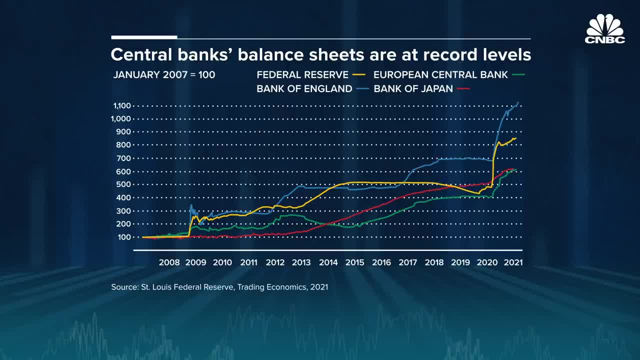 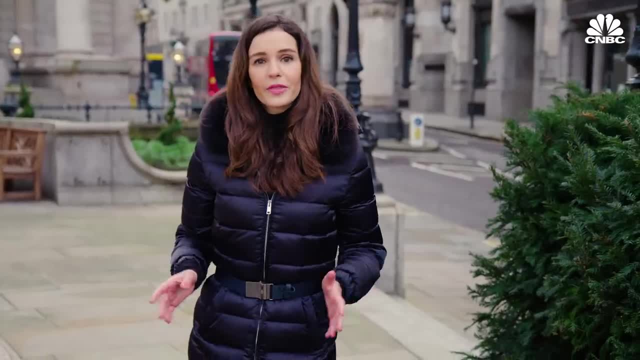 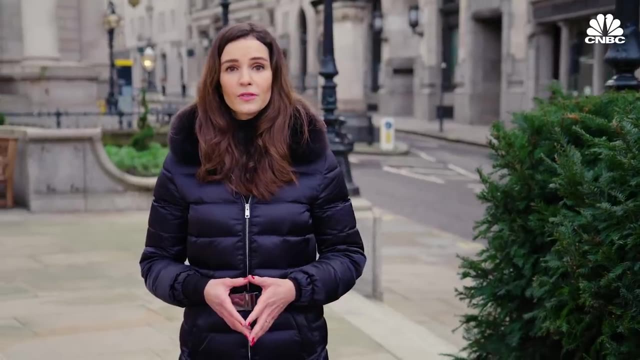 central banks have been printing more money than ever before to arrest the economic fallout from the pandemic. That's why people sometimes call Bitcoin digital gold. Many central banks are worried that the widespread adoption of these independent cryptocurrencies could weaken their control over the financial system. This could cause financial instability, especially because 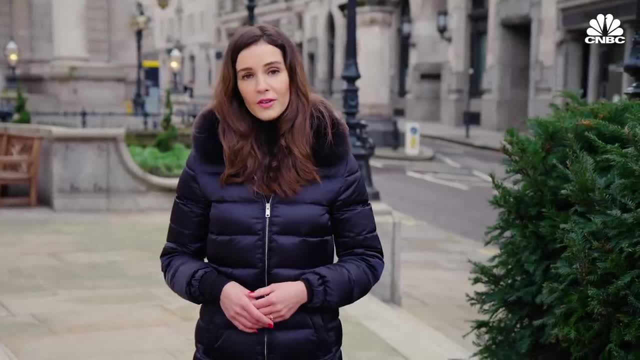 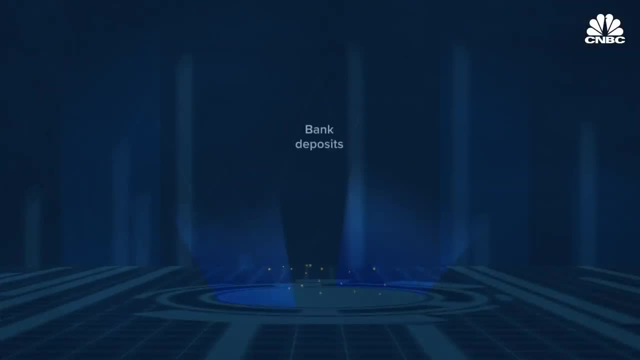 cryptocurrencies do not have the legal or the regulatory safeguards that central bank money does, So why not issue a digital currency of their own? Currently, regular bank deposits, cash and cryptocurrencies issued by the private sector, such as Diem and Bitcoin, all have a few features that make them useful. 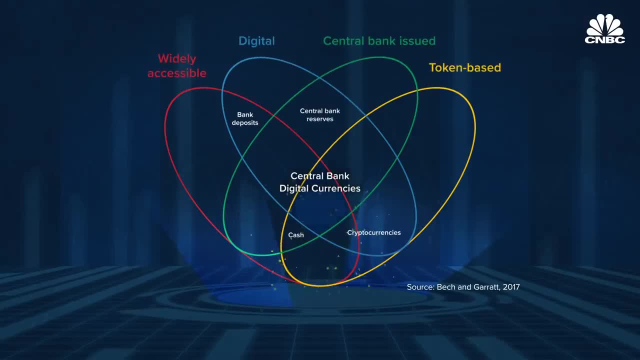 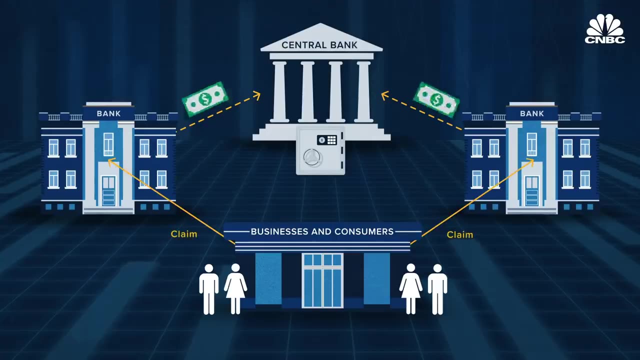 But the hope is that publicly available CBDCs would have all these desirable characteristics. Unlike your savings in a commercial bank, which rely on the bank's promise to fulfill, CBDCs are recognized by law and backed by the power of the central bank, which cannot go bankrupt. 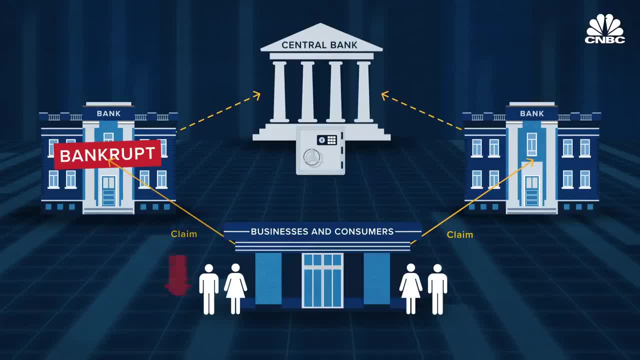 For example, if a commercial bank collapses, part of your savings could potentially be wiped out, But this wouldn't be the case for CBDCs, which could be as trusted as cash, as convenient as a payment app, yet also benefit from the same. 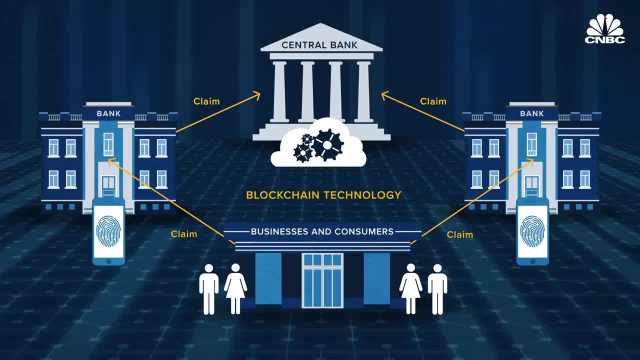 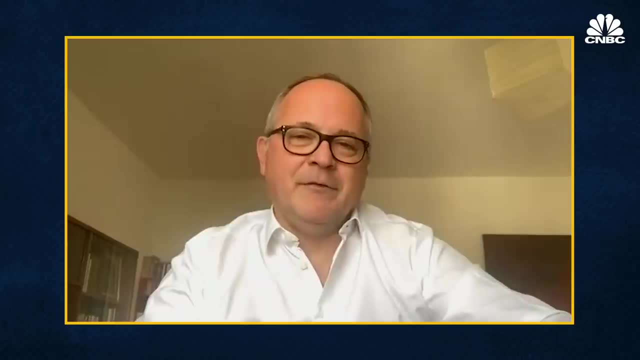 blockchain technology which underpins cryptocurrencies And, just like cash, CBDCs could be distributed through commercial banks, avoiding too much disruption to the financial system or the central bank having to deal directly with many millions of citizens and businesses. Think of banknotes, which are the closest equivalent to central bank digital. 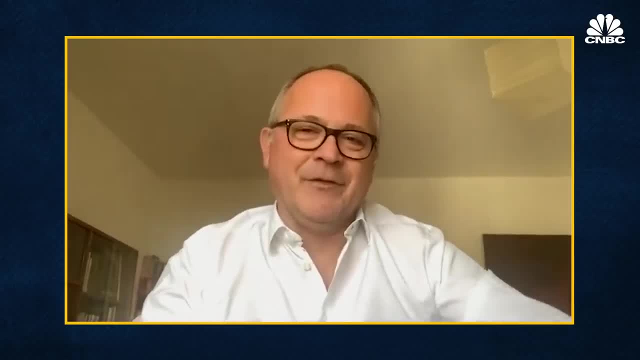 currencies that we have today. Think of banknotes, which are the closest equivalent to central bank digital currencies that we have today, Except that they're on paper. of course, This is money that is issued by the central bank and used daily in retail payments. The central bank sells banknotes to commercial banks. 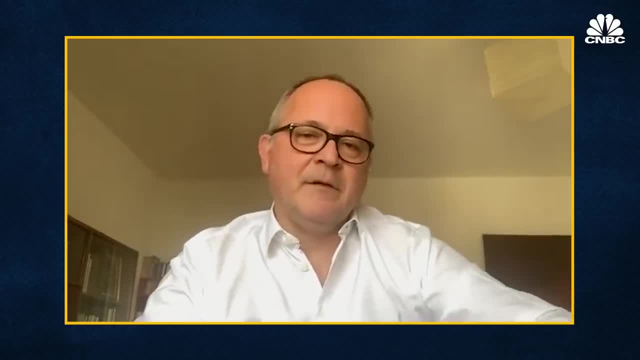 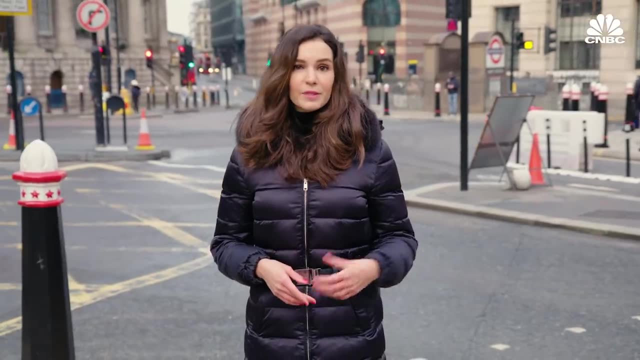 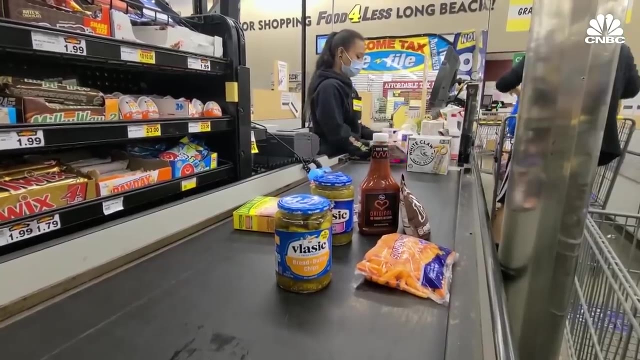 and then the commercial banks distribute banknotes through ATMs to their clients. This means that everyone could have access to this digital currency, which could bring a lot of benefits. It could make payments faster, allowing for immediate settlements and no processing delays, And it could also make payments cheaper. In the US, the aggregate cost of making 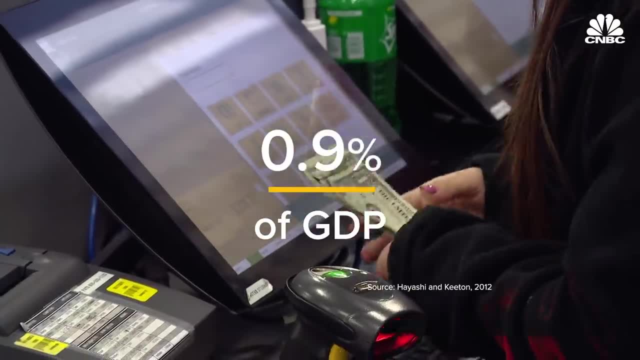 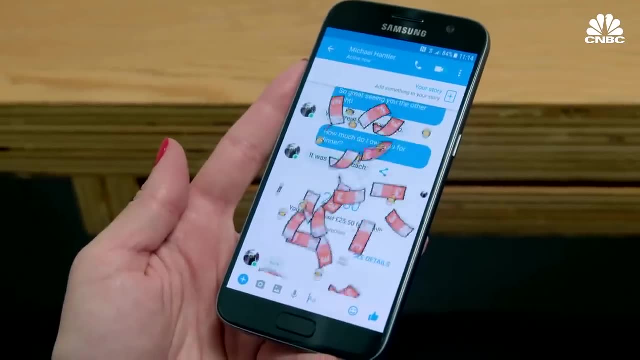 retail payments ranges from 0.5% to 0.9% of GDP. Digital currencies would reduce those costs. It also means that more people could have access to electronic payments. Currently, over one and a half billion adults across the globe don't have access to the. 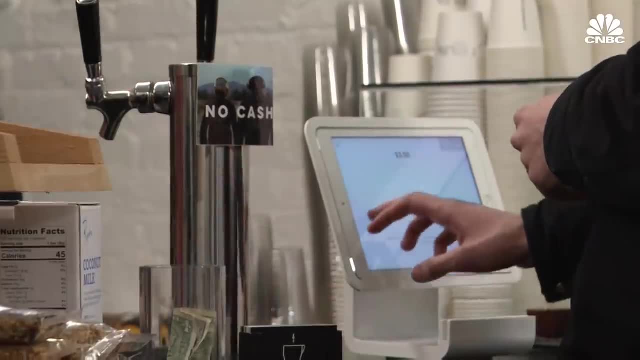 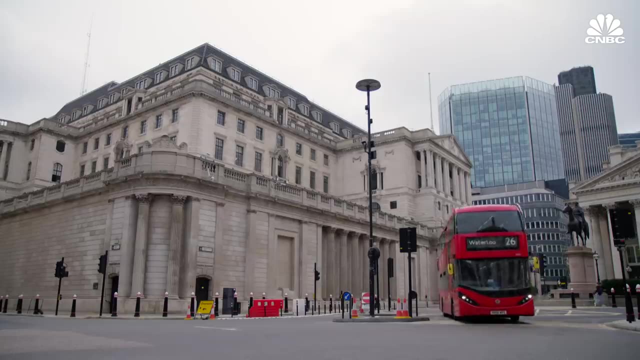 financial system, And even in an advanced economy such as the US, more than six percent of Americans don't have a bank account. Issuing digital currencies could also make it easier for governments to deliver stimulus checks or even go one step further and make targeted payments to the US. 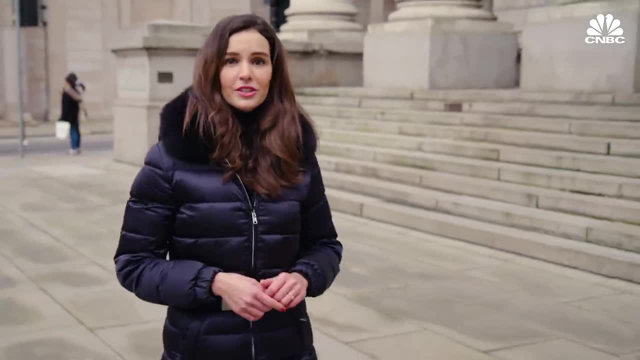 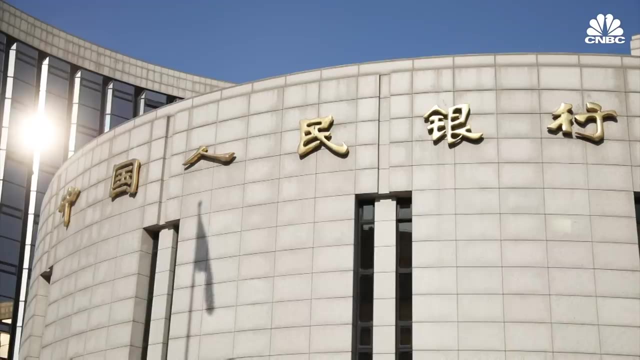 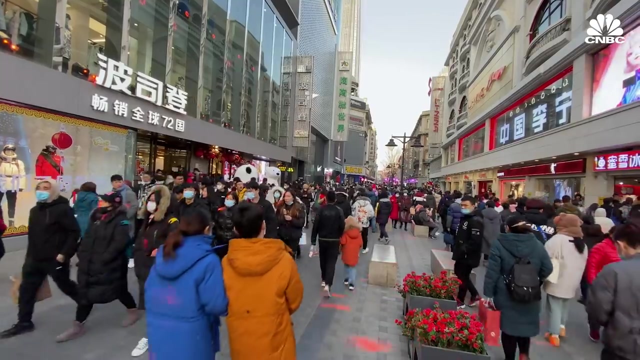 So how soon could central bank digital currencies become a reality? China is the major economy which is most advanced in its CBDC development. The People's Bank of China has been running tests of its digital currencies since April 2020, with the help of four banks in the country. Tens of thousands of consumers have already. 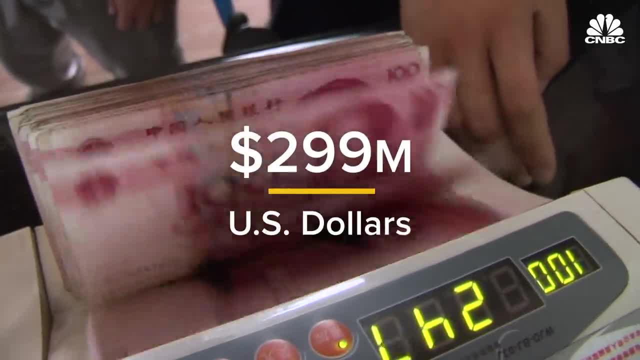 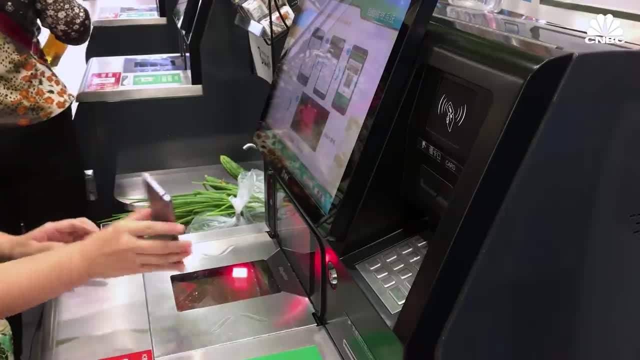 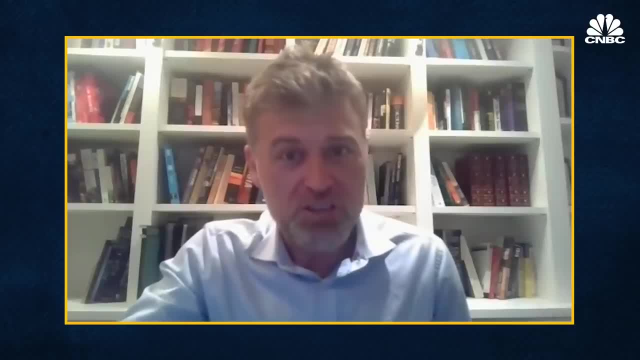 AntPay and WeChat. these are the dominant payment technologies in China and they are in the hands of Alibaba and Tencent, And if Beijing can wrest that back, then I think they will, And the way they've set up the yuan is that it will still be effectively. 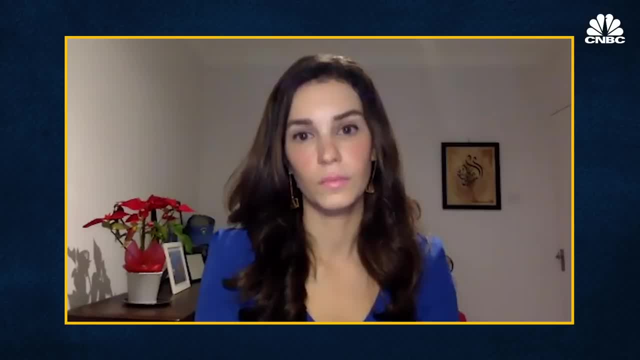 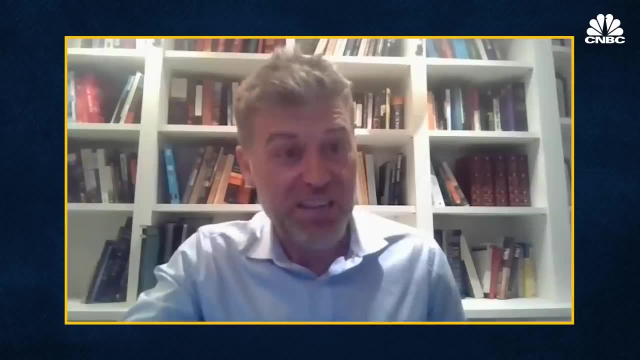 very integrated with the commercial banks, but it is effectively a direct challenge to the payment technologies. They are trying to ultimately displace them. The yuan is going to have its own digital wallet at the commercial bank And over time people will probably just find it more. 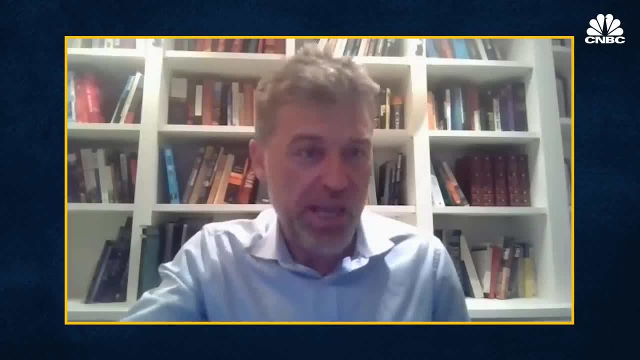 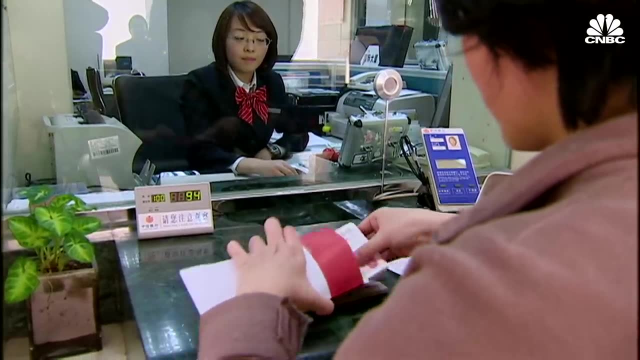 convenient to use that and thereby displacing AntPay, for example. There may also be a geopolitical consideration for China providing a mechanism to shift away from using the US dollar. There's no doubt that Beijing views the US dollar as a strategic advantage that the US has The 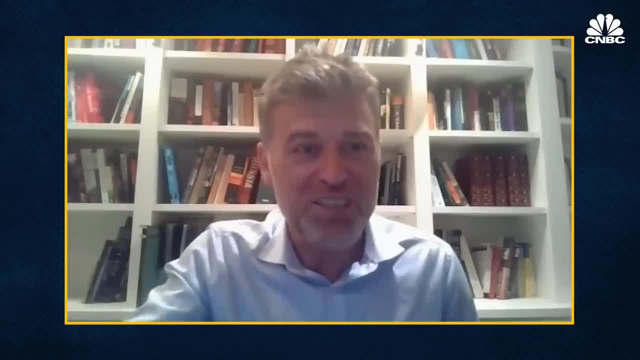 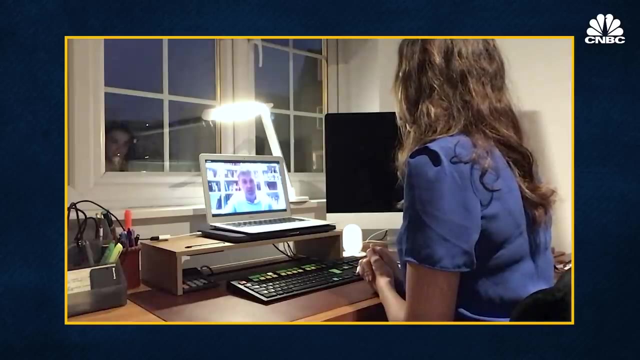 problem is that most of the real world trade is denominated and invoiced in US dollars And China sees this and it's very hard for them to sort of push renminbi into the global financial system, the global trading system. But they're trying. But if they had a digital currency, that would be. 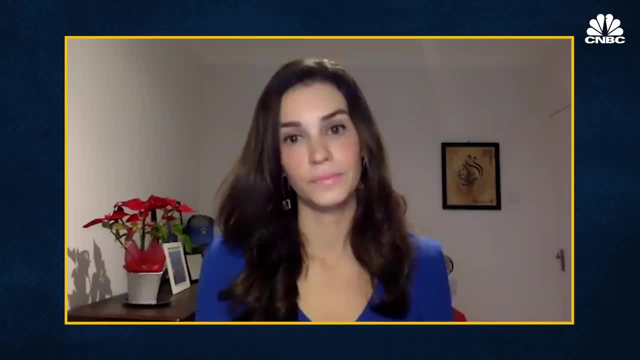 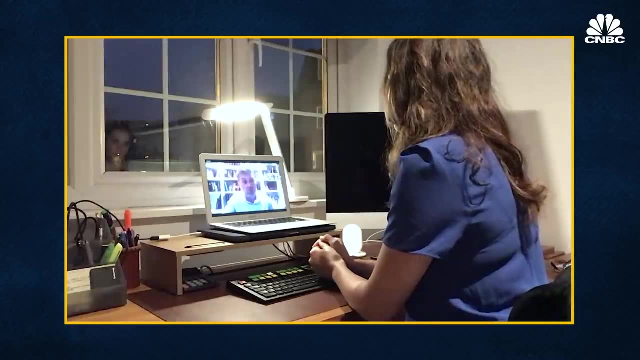 potentially a really fascinating angle. So you can see if it's got a technological advantage, that perhaps this is a way for people to think about the renminbi in a different way and perhaps, you know, ultimately start to chip away at the hegemonic status of the dollar. 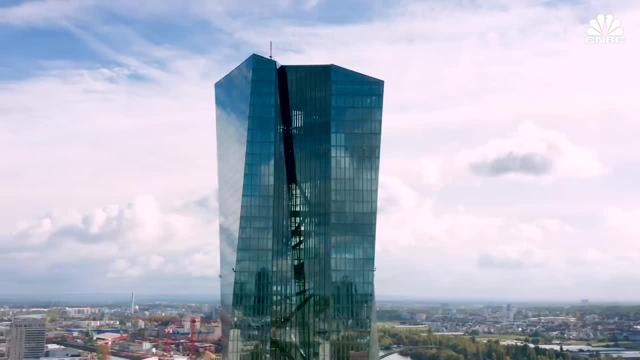 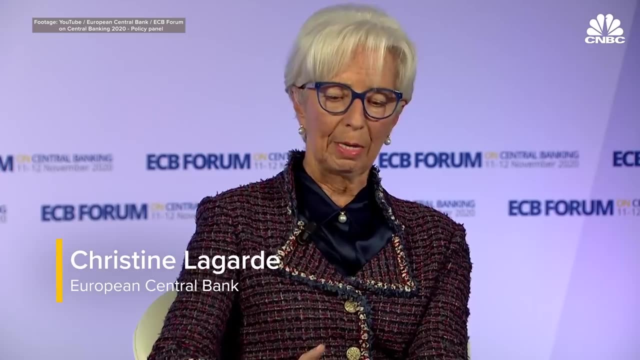 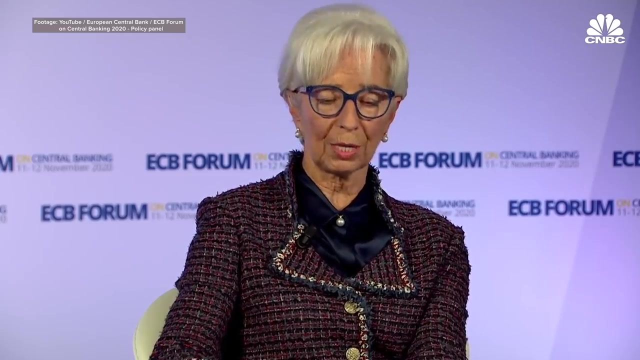 But it's not just China. The European Central Bank has plans for a digital euro, although it may be a few years before it is available. We are going to have to address all the issues of anti-money laundering, financing of terrorism, privacy of users and all the information. 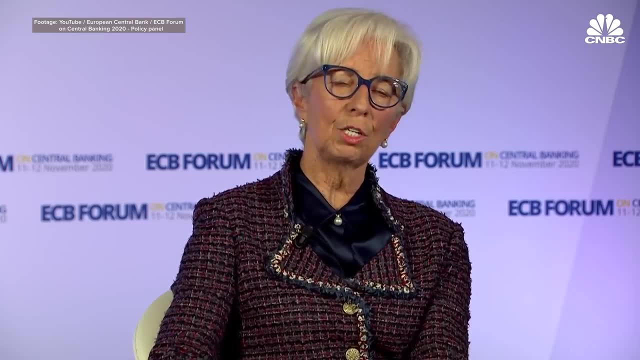 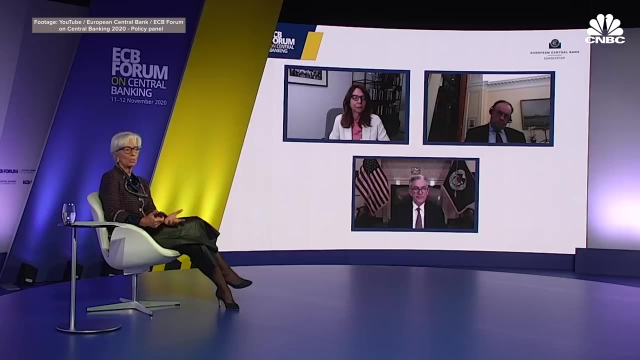 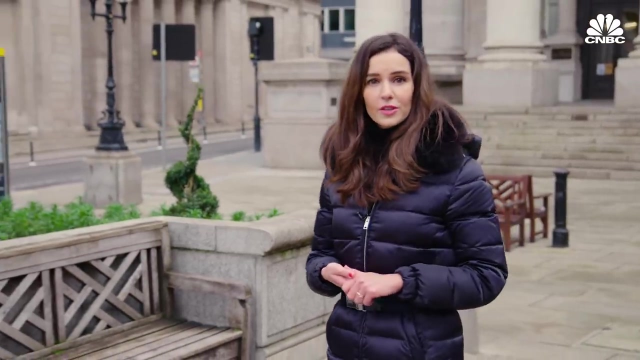 the appropriate technology that will carry that digital currency. And this is, you know, a project that will probably take us two, three, four years before it is, before it is launched. This has got people wondering whether issuing a central bank digital currency could interfere with the effectiveness of monetary policy. 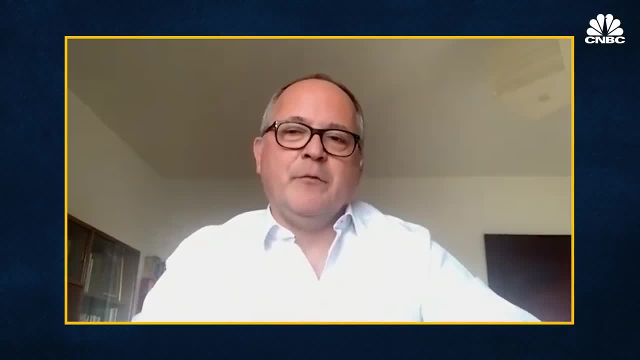 Central banks have addressed CBDC so far is really as part of a payment discussion. That's a discussion for monetary policy committees, for the ECB Guarantee Council, whether they want to use CBDC or not. But it's too early to have that discussion. 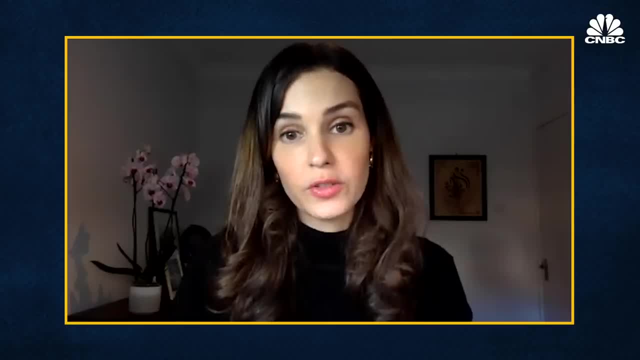 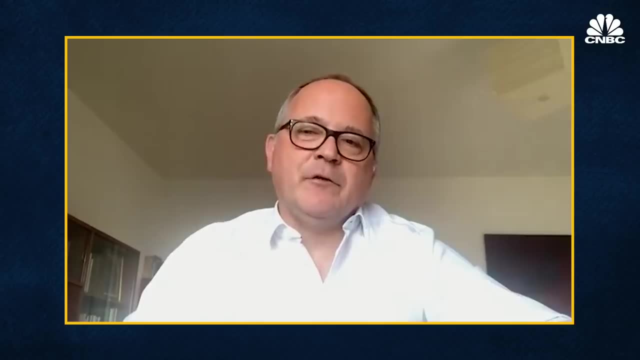 But theoretically, if the central bank wanted, they could also pass on negative rates to the holders of central bank digital currencies- Think of CBDC as being these a few years ago. you know the future of banknotes. Banknotes do not bear interest, And so if you. follow that line of reasoning, then CBDC should not bear interest. And if you want CBDC to bear interest, then you're creating something different. A lot depends on how much people would use CBDCs, and no central bank wants them to completely replace traditional cash, but rather to complement. 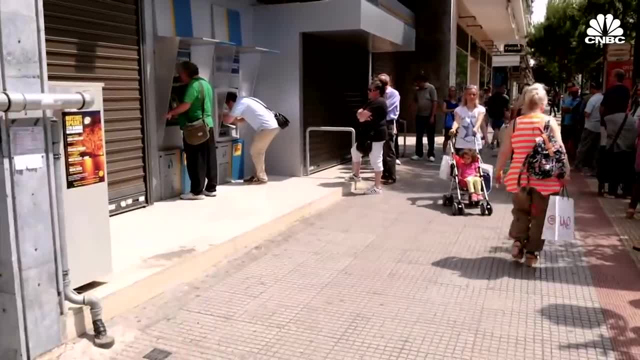 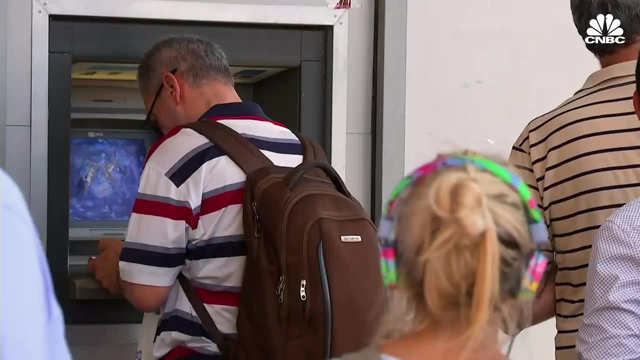 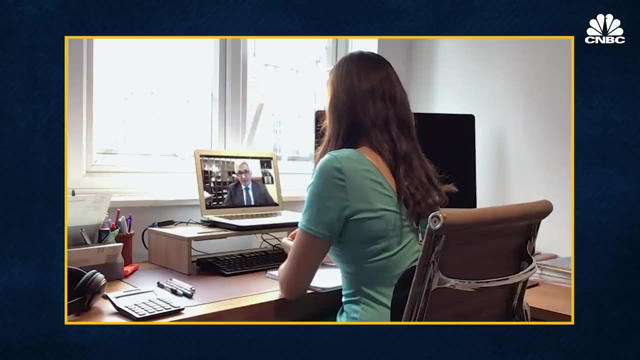 it. One risk associated with CBDCs is that in an extreme situation, such as after a financial crash, banks would have to withdraw their deposits from commercial banks and opting to store their money in digital currencies backed by the central bank. Trouble would be if CBDC would replace bank. 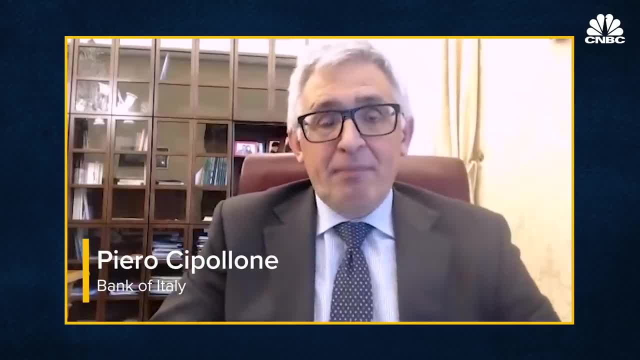 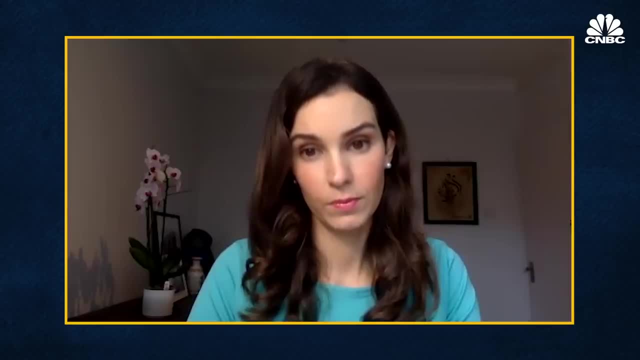 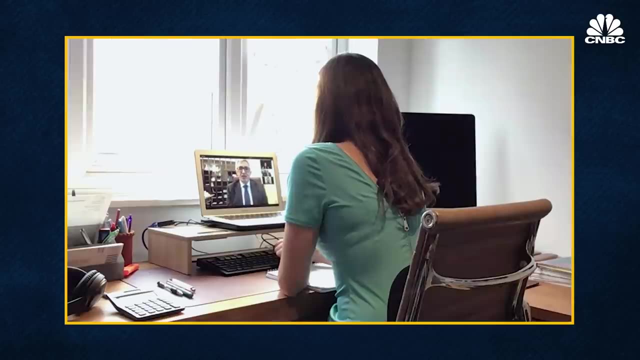 deposits in a large amount, Because then what happens is that savers could shift their saving from bank account to CBDC. Then banks could have a problem for funding. This might have an effect on the financing of the whole economy. People can shift that they're saving from a bank. 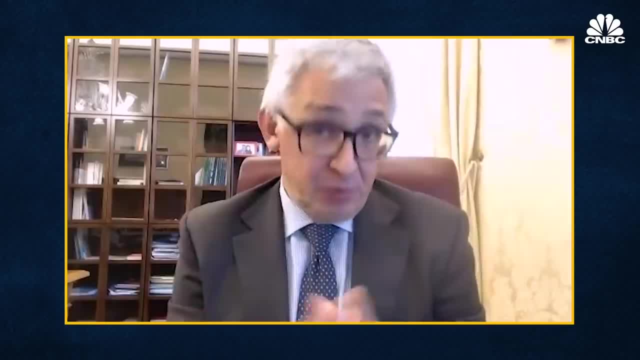 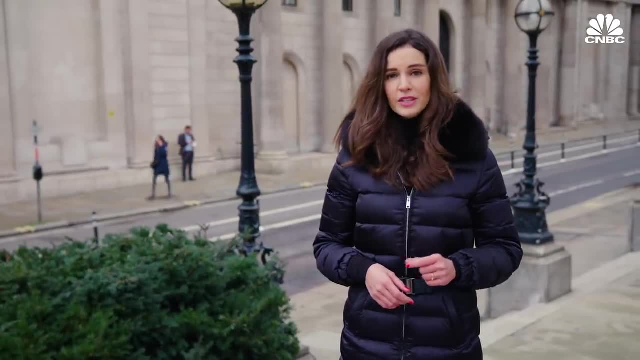 account to CBDC just with that click, And this would be very dangerous, obviously, As we move towards a more cashless society, will central bank digital currencies ever become as trusted and as convenient as banknotes? Quite possibly, though it may take months, maybe even years. 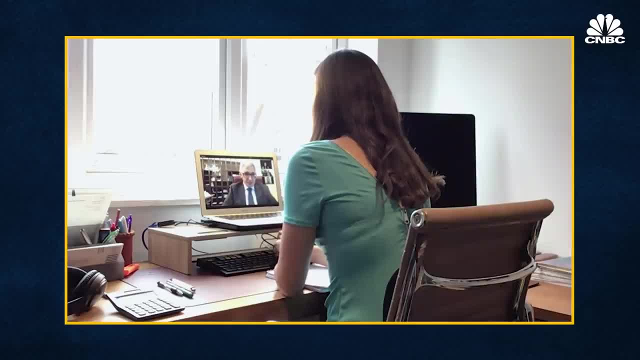 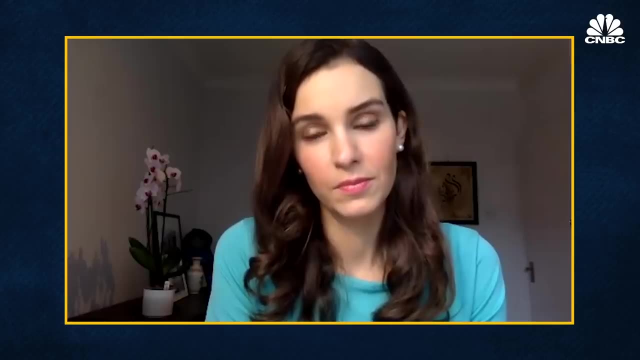 The trust in private money is built on the trust on the currency and the fact that behind that there is a central bank which has tools to keep the value of the currency. We have to buy this trust And that's why we need to stay into it, into the economy And the way to stay into the economy. 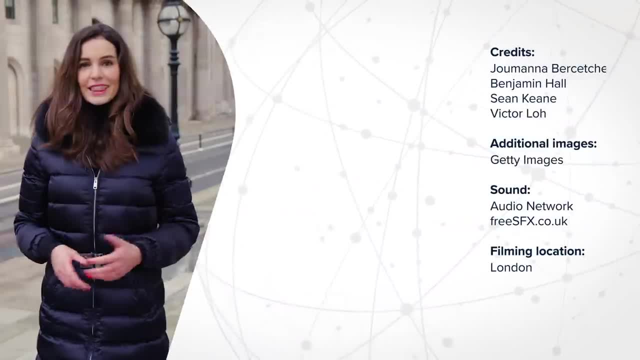 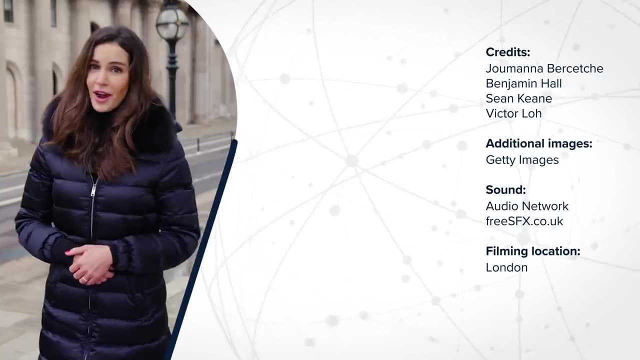 is to make sure that people trust us. Thank you for watching. Would you ever use a central bank digital currency? Let us know in the comments and don't forget to subscribe. 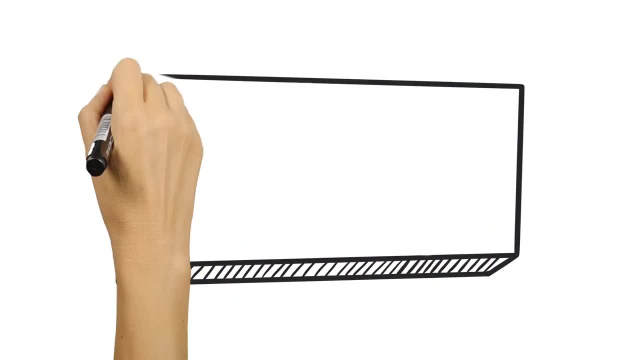 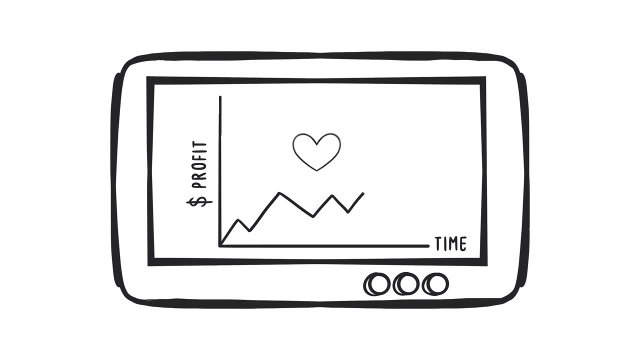 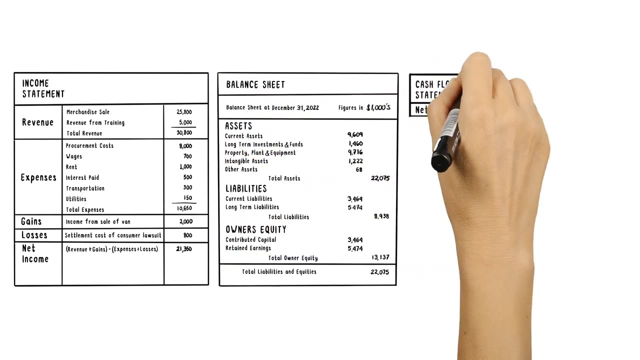 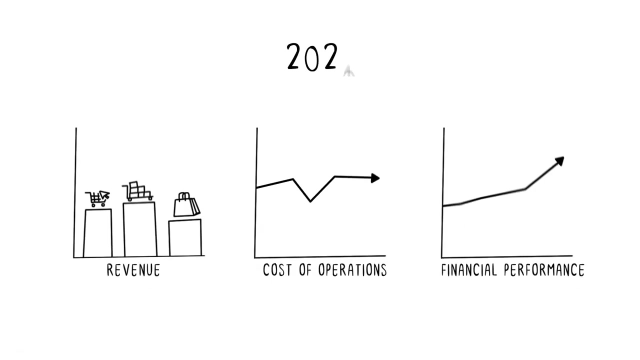 What is a financial statement? Financial statements detail a company's financial health and performance at a specific point in time. Made up of three standard reports- the income statement, the balance sheet and the cash flow statement- financial statements convey how a company generates revenue, how efficiently it operates and whether it's making or losing money. 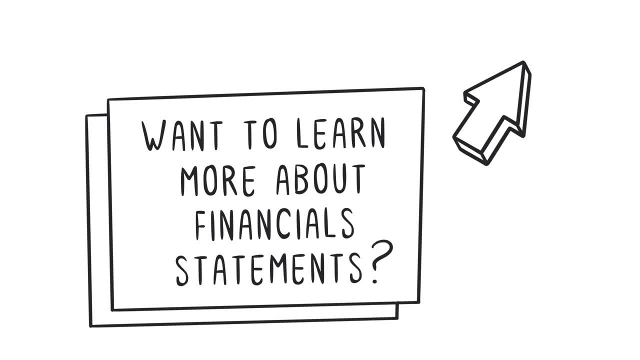 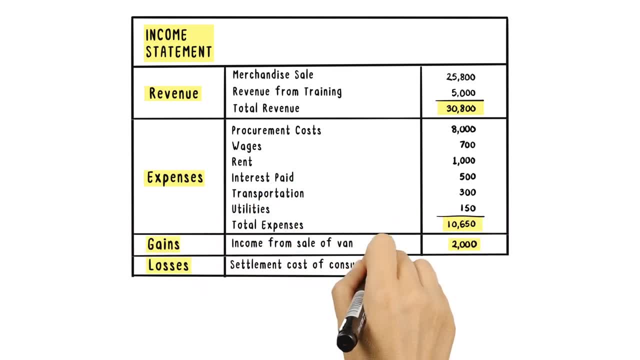 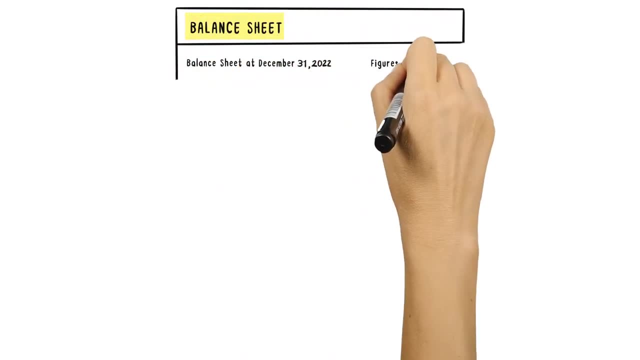 Want to learn more about financial statements? Click the link in the top right corner. The income statement shows how much money a company earned from its core operations, as well as financing activities and investment gains or losses. The balance sheet captures the value of a business's short and long-term assets. 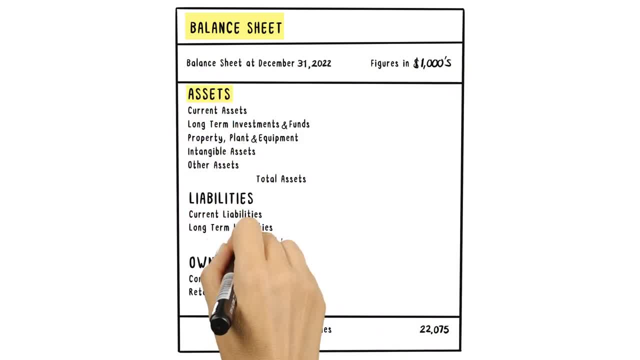 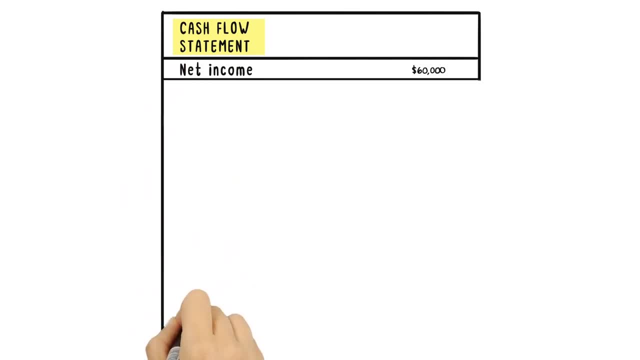 including tangible items like cash, inventory and equipment, as well as intangible items like patents, trademarks and goodwill. The cash flow statement indicates how much cash came into a company during a report and how much money it earned. The cash flow statement shows how much cash was spent during a reporting period and how much cash was spent. 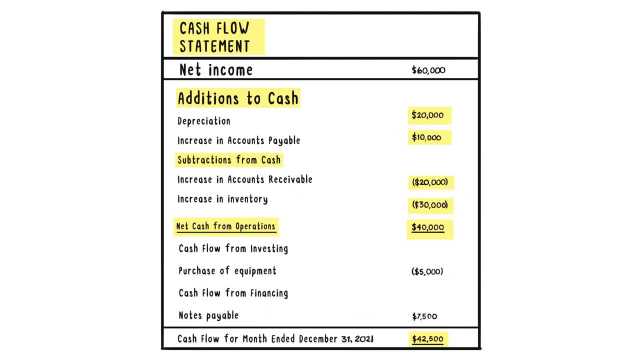 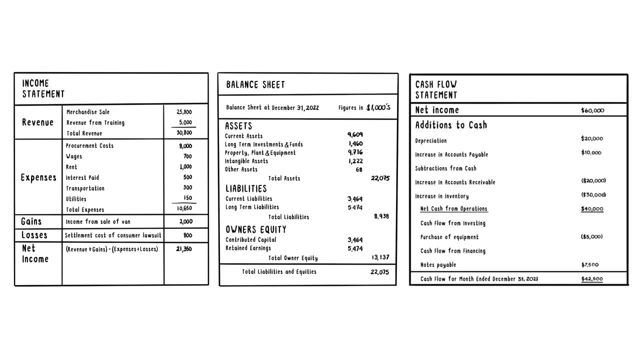 Like the income statement, a cash flow statement conveys where the money is coming from and what it's being spent on. Individually, these documents only tell part of a company's financial story, but if used together, it can help internal and external stakeholders. 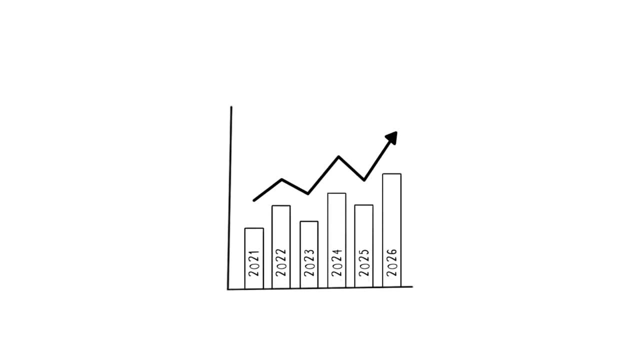 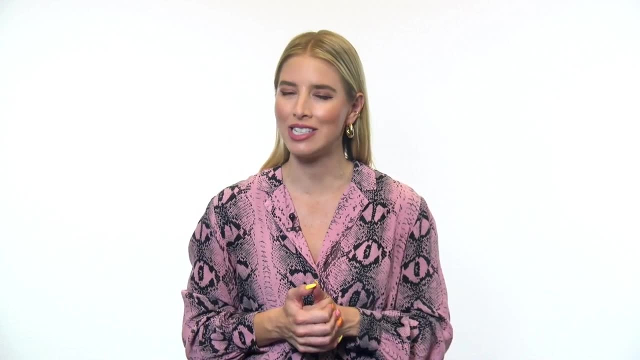 determine whether a company is financially stable or headed for trouble. The cash flow statement indicates how much cash is dedicated to an organization, which is what we'll look into in a minute. Once you know the sieve, make sure you remember to include bank accounts.